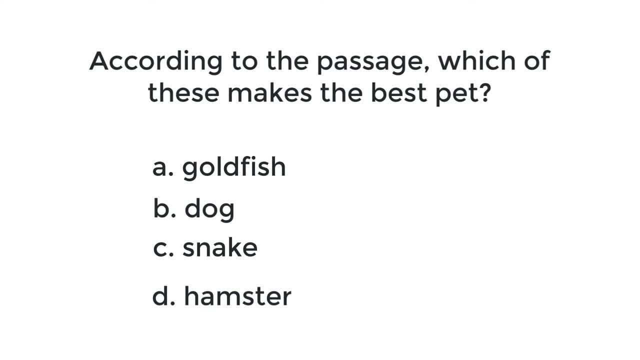 Multiple choice questions consist of the stem, which is the opening, a problem to be solved, a question asked or an incomplete statement to be completed, And the options are the possible answers that you, the examinee, can choose from, But the correct answer is called the key and the incorrect answer is called distractors. 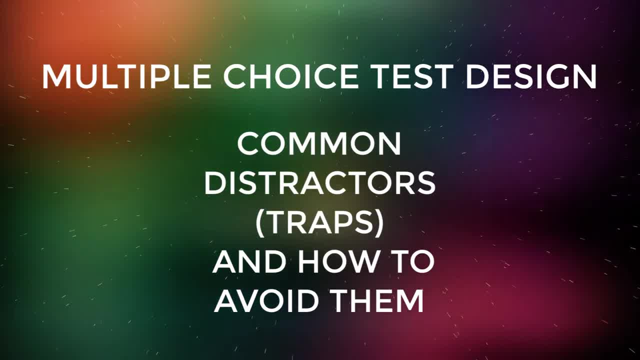 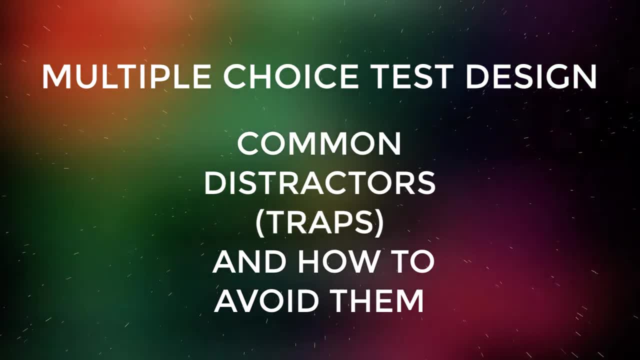 In this section we are going to see how distractors are designed on multiple choice tests And how to avoid these trap answers. Notice how they are labeled: distractors and I like to call them trap answers. Remember that they are written in a way where they seem plausible and reasonable. 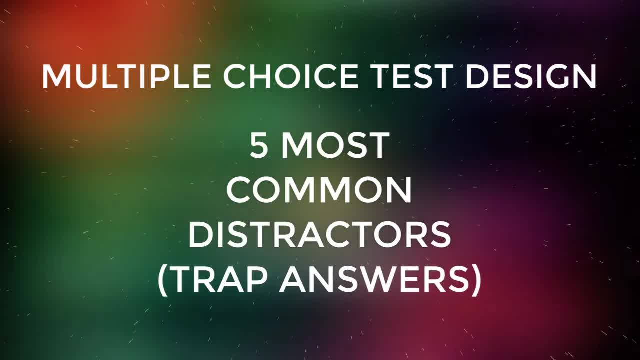 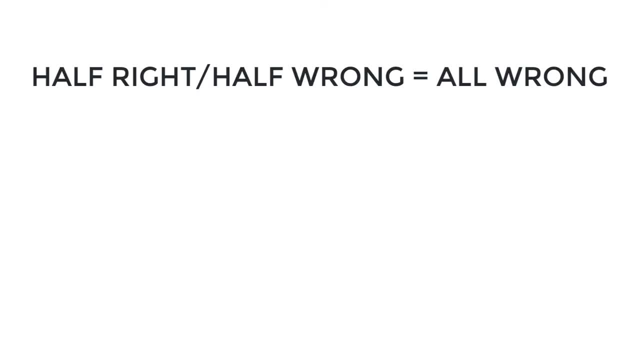 There are five trap answers that are common in multiple choice tests. The first one is a half right, half wrong answer. In this type of distractor, the details from the passage are twisted or distorted and they are no longer correct. There may be some element of truth or fact. 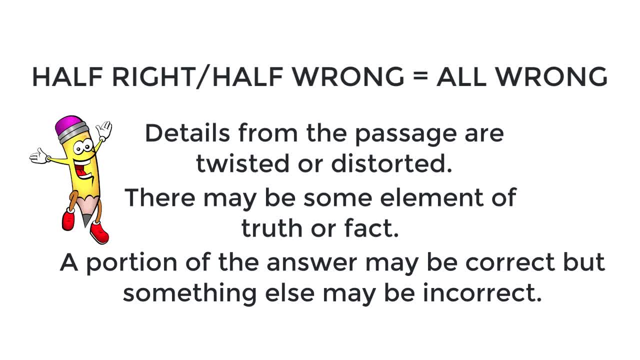 A portion of the answer may be correct, but something else may be incorrect. Remember, if a portion of a multiple choice distractor is just a tiny bit wrong, it's all wrong. Let's look at this example. Wolf characterizes the moment of transition as both: 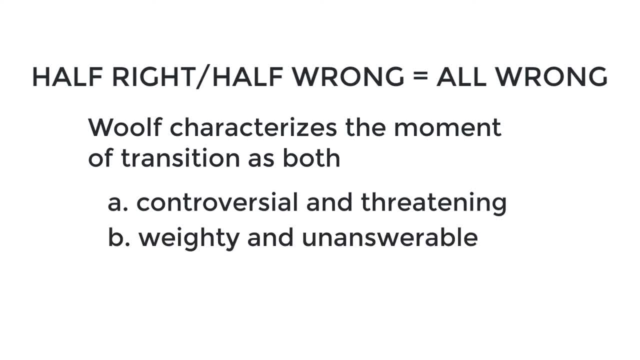 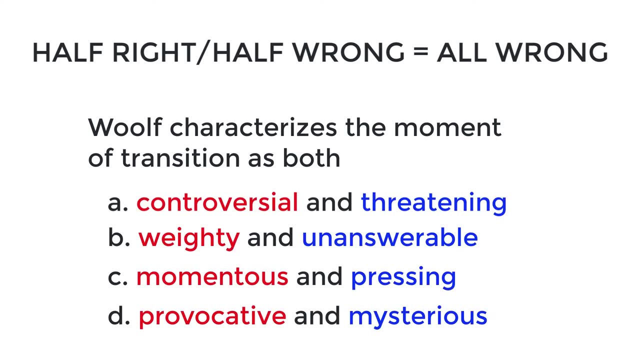 A- Controversial and threatening, B- Weighty and unanswerable, C- Momentous and pressing. and D- Provocative and mysterious. You will see that for each choice we have two possibilities. If any of the possibilities are incorrect, we strike out the entire choice. 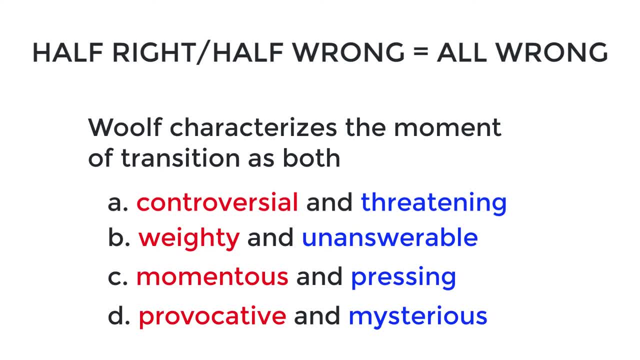 So, for example, let's say that for letter A, controversial would fit the passage, but threatening would not. so we strike out. letter A: Weighty may fit the passage, but not unanswerable. Momentous fits the passage. Pressing fits the passage. 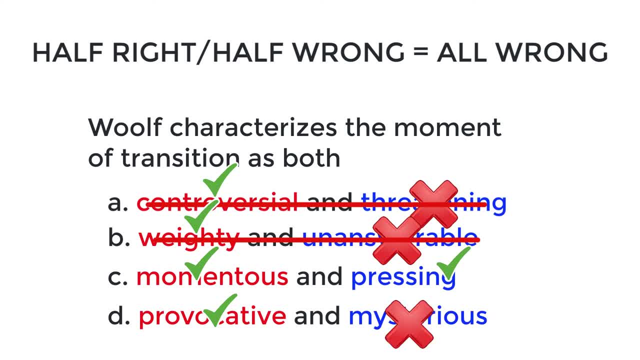 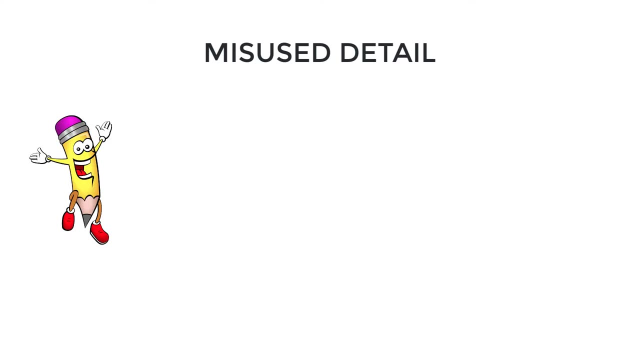 Provocative may fit the passage, but not mysterious. so we strike out letter D. So the correct answer is letter C: momentous and pressing. Let's go on to the second type of trap answer, and this is the misused detail. 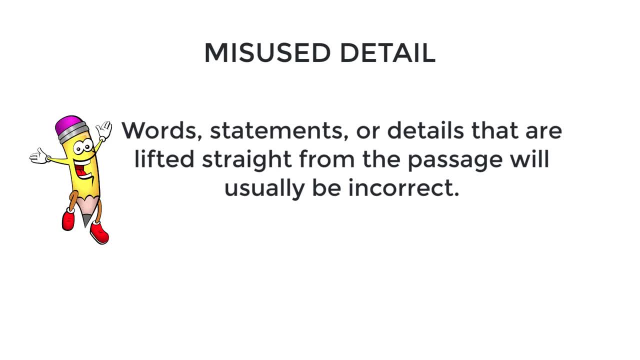 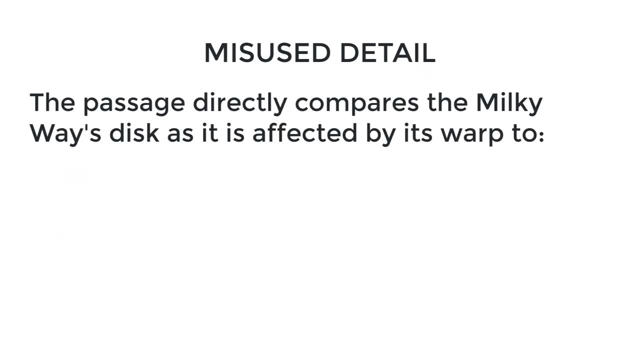 Word statements or details that are lifted straight from the passage will usually be incorrect. These will be in word-for-word format. The more the wording resembles the text, the likelihood of being incorrect increases. Let's look at this example. The passage directly compares the Milky Way's disk, as it is affected by its warp, to 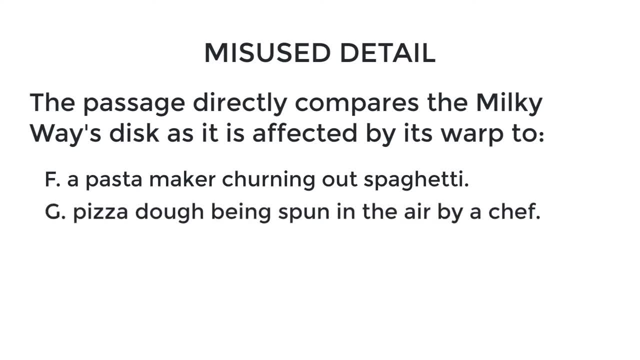 F- A pasta maker churning out spaghetti. G- Pizza dough being spun in the air by a chef. H- A thin crust pizza balanced on top of a plum. J- Two figure skaters coming together for a combination. spin All of the choices in this multiple choice question. use details lifted straight from the passage. 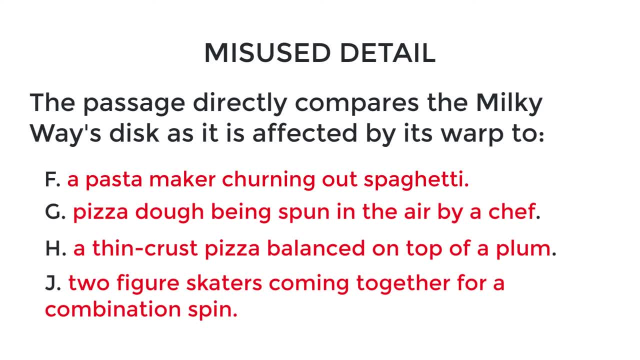 In other words, the language in all of these choices comes from the passage. So you have to be very careful, because only one is going to be the correct answer. In this case, the correct answer is G Pizza dough being spun in the air by a chef. 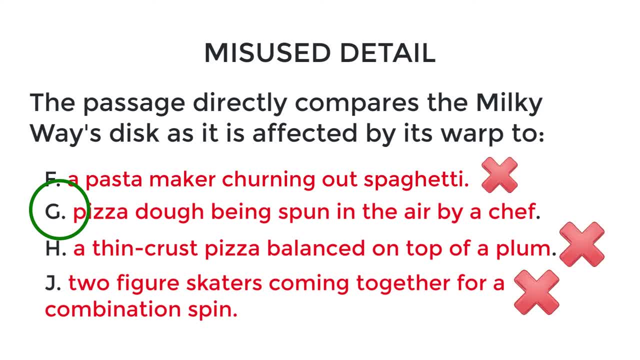 But letters F, A and G are incorrect. F, H and J all used word-for-word language lifted straight from the passage, So you must be careful not to fall for this trap. I want to make one observation about the answer in this question. 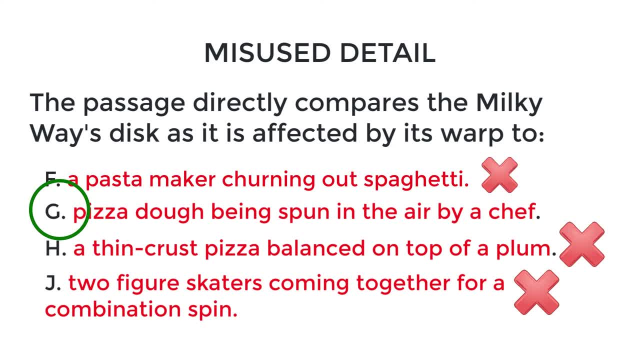 Typically, the correct answer does not use language straight from the text. Most often, the correct answer is paraphrased. We will learn more about this in the lesson. Let's go on to the next type of choice, The trap answer. This is the out-of-scope answer. 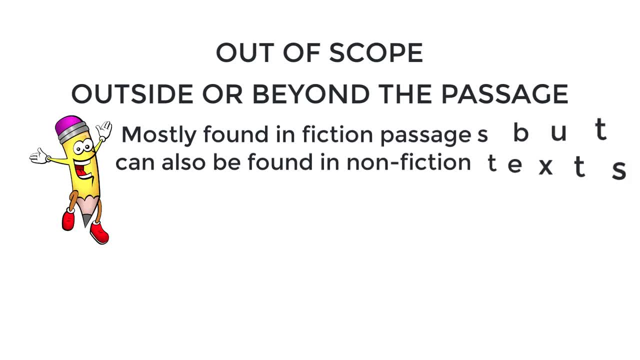 This type of answer is typically found in fiction or narrative passages, but it can also be found in expository or non-fiction text. This distraction plays on your own background, knowledge, your world views, your personal ideas and biases. This interpretation will make sense, but is not supported by the passage. 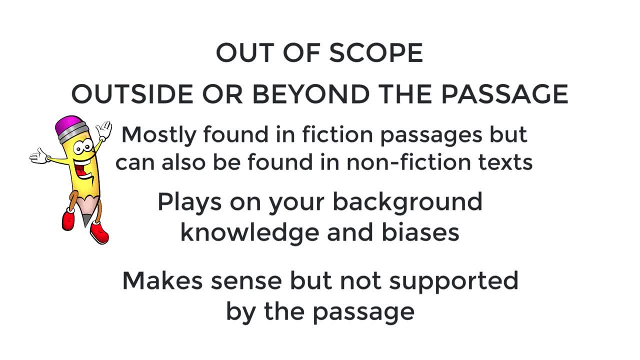 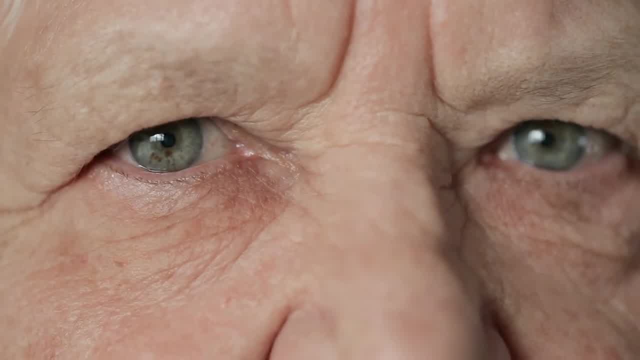 because it was never stated explicitly or implicitly. Let's think about a passage about an old woman who has lived in the woods for over a hundred years. She has not had any human contact for all this time. She claims that she has been free of the constraints and the trappings of structured society. 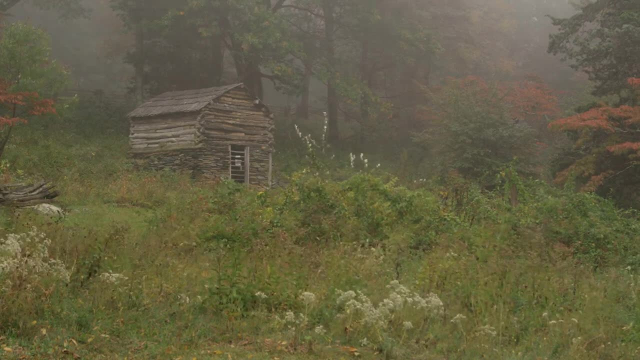 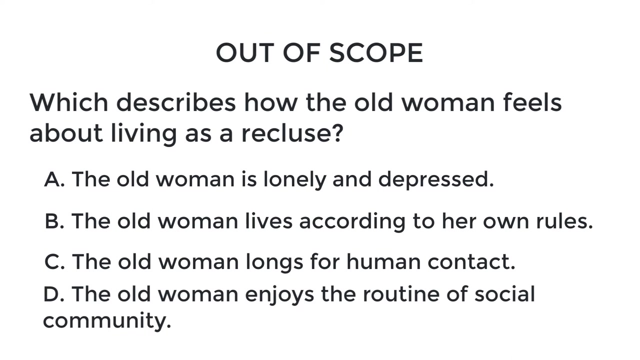 Now let's say that the question may ask you how the old woman feels about living as a recluse, And in one of the choices it states that the woman feels lonely. Now this is a totally plausible answer, because someone who hasn't had human contact in a long time may be lonely. 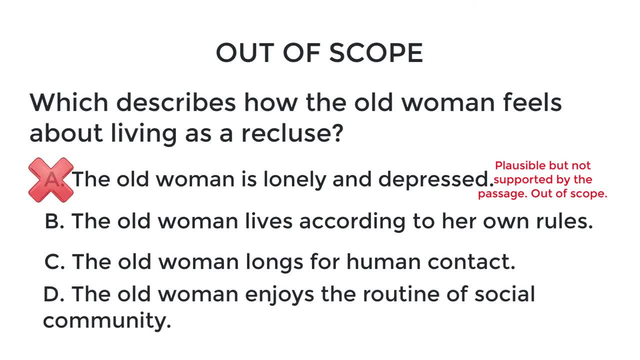 This is a totally plausible answer, because someone who hasn't had human contact in a long time may be lonely. This is a totally plausible answer, because someone who hasn't had human contact in a long time may be lonely. However, the passage never stated that the old woman longed for human company. 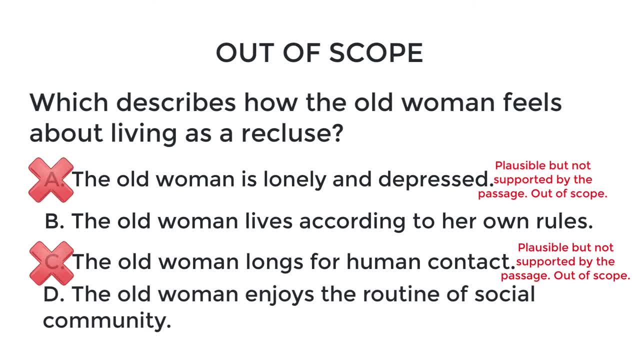 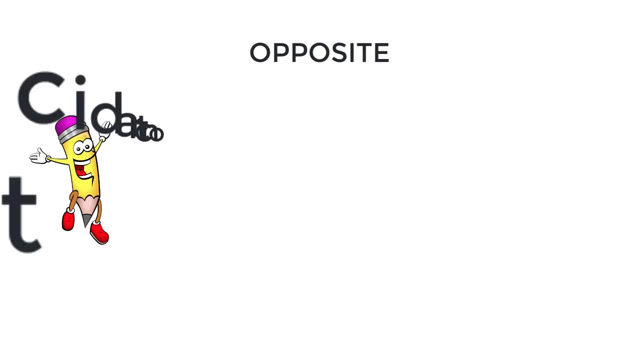 Therefore, you cannot infer that she is lonely. Your thinking is out of scope, It is outside the passage and you've fallen for the trap. The next type of trap answer is the opposite. This type of distractor contradicts the information in the passage. 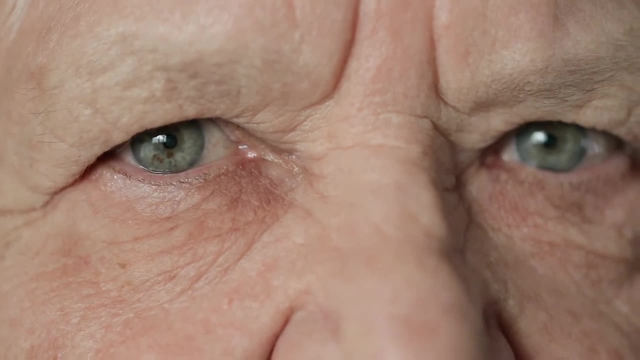 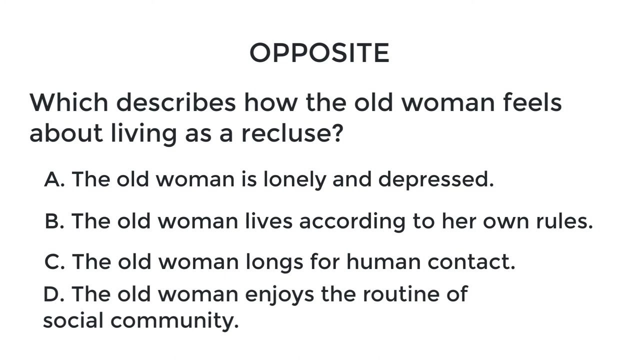 Let's go back to the story about the old woman. Again, if the passage says that the old woman felt free of the constraints and the trappings of structured society, an opposite type of answer may say that she enjoyed the routine of social community. 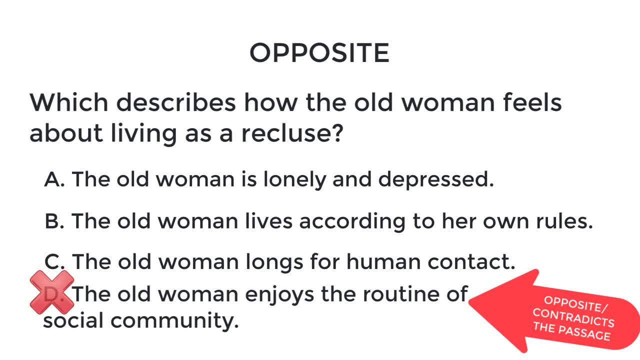 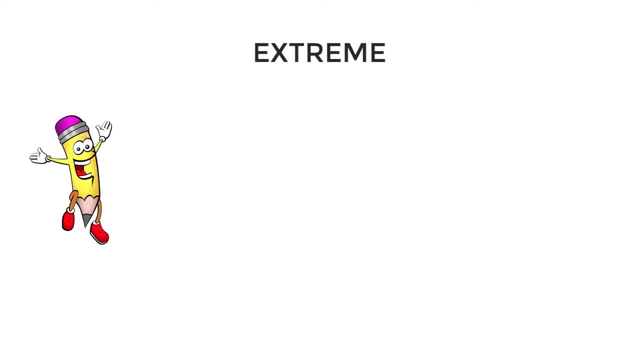 Well, this is obviously an opposite, because she does not enjoy the routine or the customs of structured society. And the last type of trap answer is the extreme trap answer. These type of distractors are based on absolute positions. These choices are almost always incorrect. 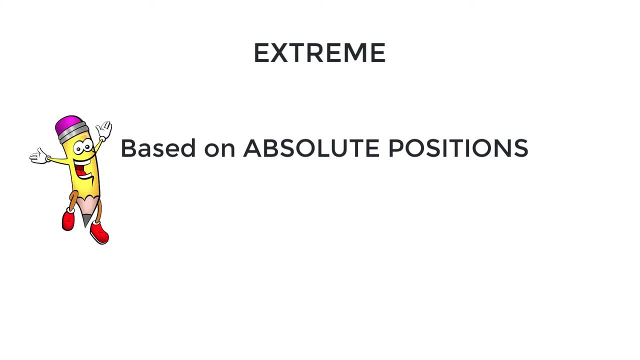 Notice that I said almost always, Because if I said always incorrect, I myself wouldn't be making an extreme assumption. So they are almost always incorrect, unless stated in the passage. Be wary of distractors that have words such as always, never, all, none, best, worst or any kind of absolute. 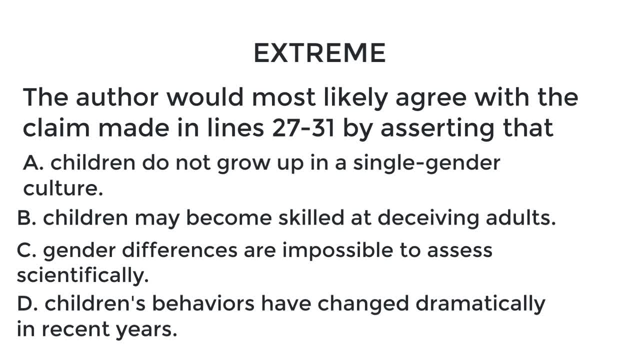 Let's look at this example. The author would most likely agree with the claim made in lines 27 through 31 by asserting that: A- Children do not grow up in a single gender culture. B- Children may become skilled at deceiving adults.